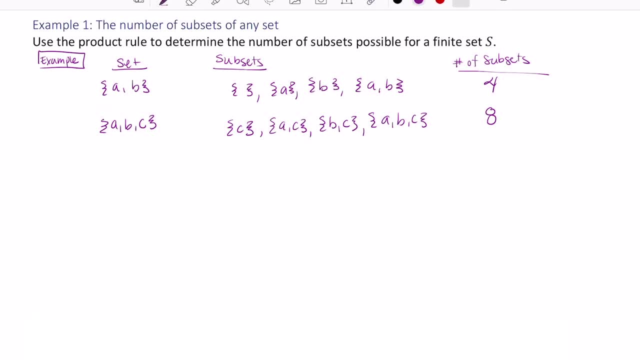 Pause the video and see if you can figure out how many subsets exist for A, B, C, D. So take a moment and see if you can count the number of subsets for a set containing A, B, C, D, That is, a set containing four distinct elements. 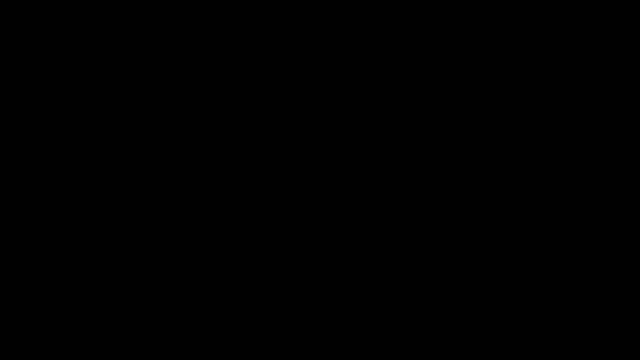 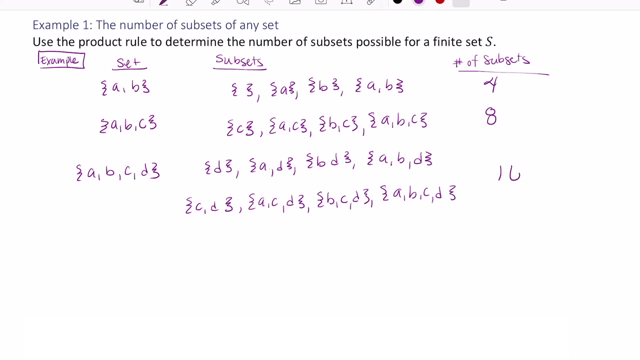 How many subsets total will I have? All right, you should have figured out that we have 16 total subsets now And they're all visible here. So this set has all of these as subsets. Now let's rewrite this: This is 2 times 2.. 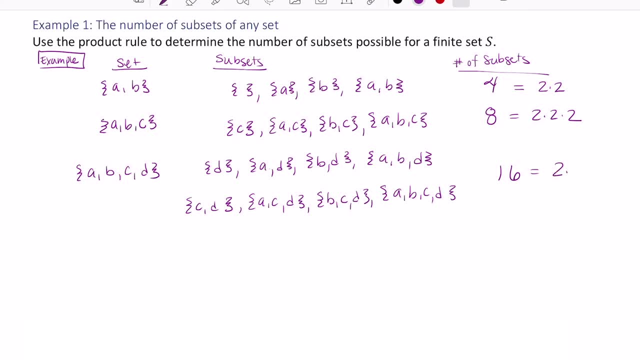 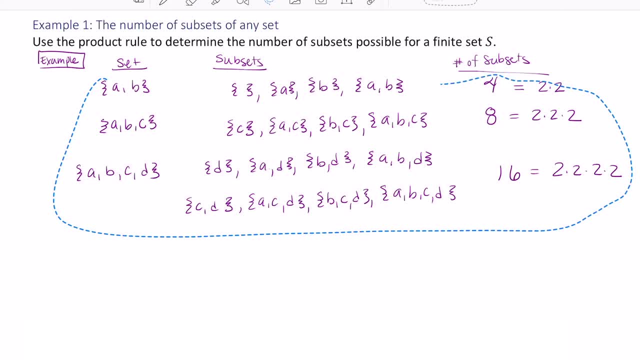 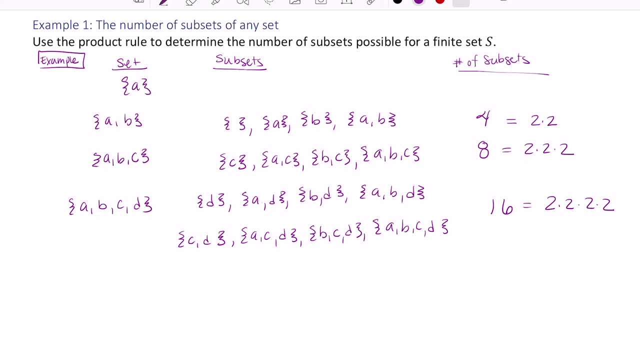 Hmm, Actually, let's add a top row here. Maybe this will help you see what to do with the product rule. What if my set was just A? The only subsets I have are what? A and the empty set. So this set has A and the empty set as a subset. 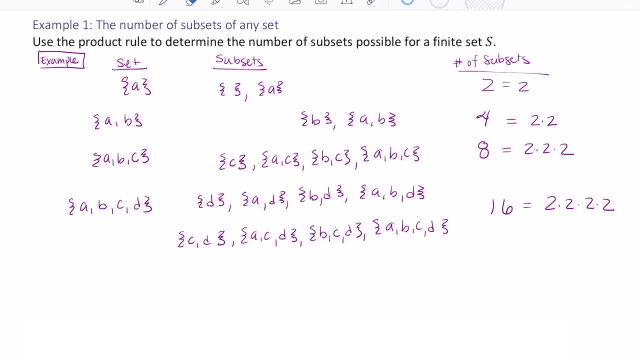 So two total subsets. So, if you notice, for every single element we add into our set we're doubling the number of subsets, Since for each element we add we have to take into consideration the subsets we already have and include the new element. 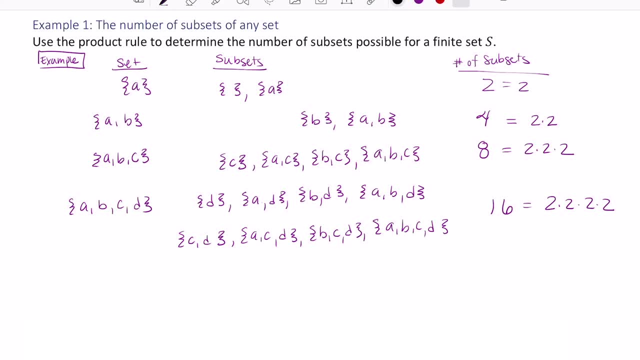 in all of the preexisting subsets. So that tells me that if a finite set, S, has cardinality N, then S has 2 to the N number of subsets. Let me